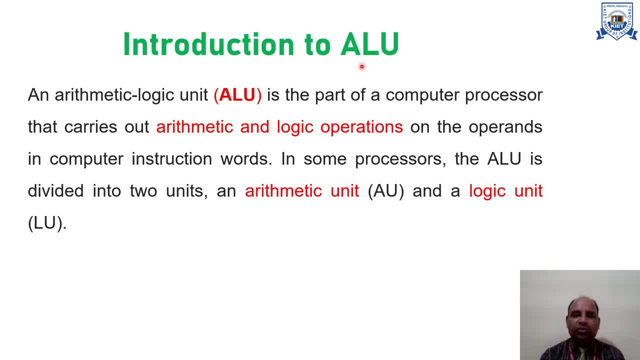 Dear all, as you know that ALU stands for Arithmetic Logic Unit, Arithmetic Logic Unit. basically, it is a central part of any processor inside the computer and it is used to carry out the arithmetic logic operation Up to this moment. I hope you all are clear. what are the different? 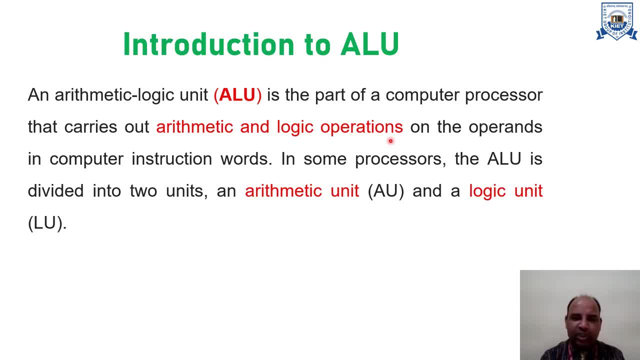 arithmetic and logic operations For your kind information. at this moment, I would like to tell you that ALU is responsible for addition, subtraction, multiplication, division. These are the arithmetic operations and logical AND logical OR logical, NOT logical OR logical EXOR, logical EXNOR. These are the logical operations, what we all have studied. 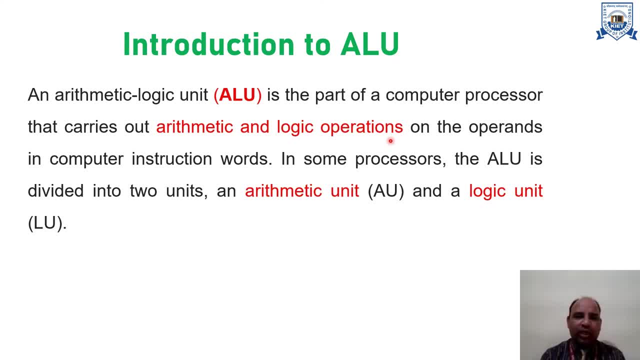 so far in this particular course. So your ALU is responsible for these operations and also it is also responsible for some shift operations, What we discussed in the previous class. they are very important when we are having a requirement for changing the values inside a register, Just to change the meaning or just to change the meaning. 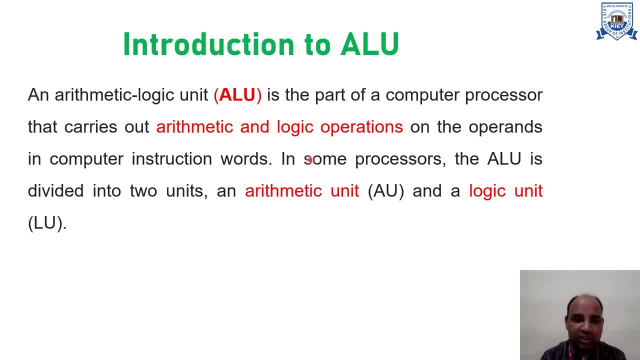 of the control signal or to change the status of a register. So they are also very, very important part within the ALU. So in nutshell I can say that your arithmetic logic unit used for arithmetic operations- what I still just told you a couple of minutes earlier- and for the logic 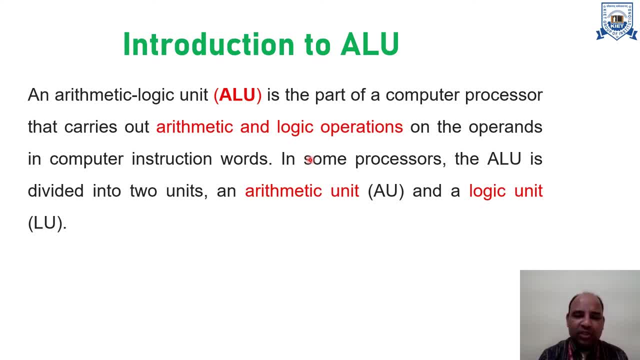 operation and the shift operation. That is what it makes the ALU, which is a very, very integral part of any processor. So now we move further. In some processor the ALU is divided into unit. In some processor- or you can see, in older processor, I can say that it is divided into two units. 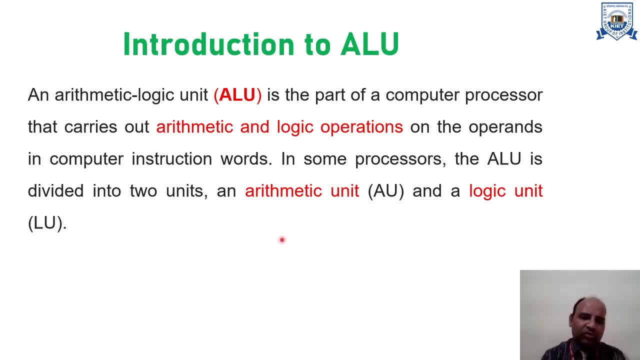 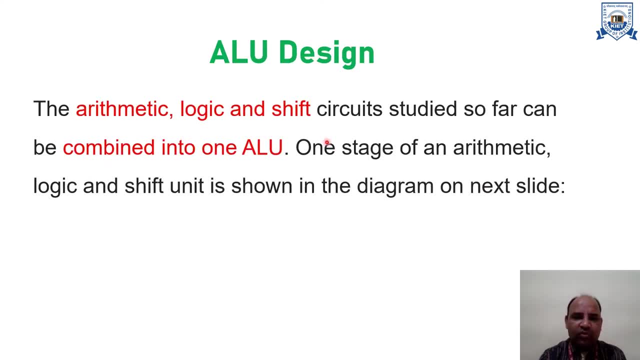 that is, arithmetic unit AU, and a logic unit, LU. Otherwise, in general, it is a combined unit which is known as the ALU. Now we move on to the next slide, the designing of the ALU. As you know that I am telling you. 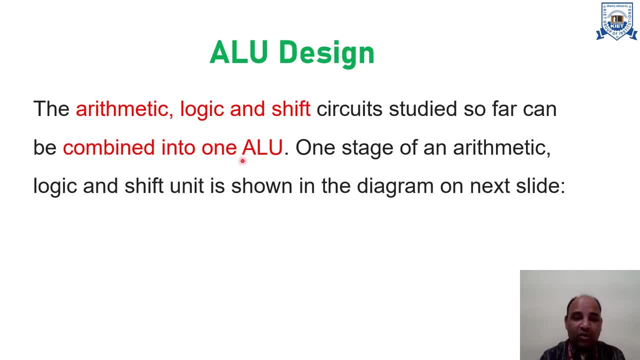 repeatedly. it is a very, very important and central part of any processor. So it requires a lot of effort designing thinking and really a tedious task, the designing of the arithmetic and logic unit, because your entire system ultimately at the hardware level, at the lowest level, 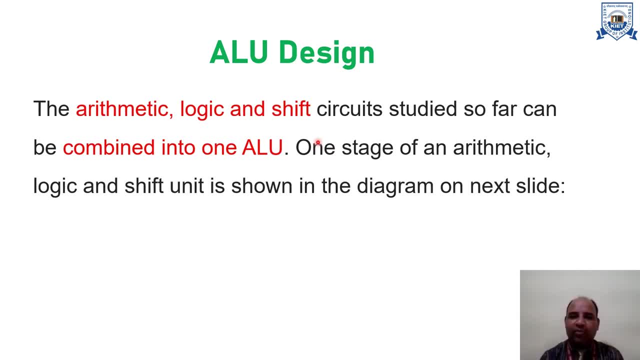 it does not matter in which language or which platform you are working as a user on your computer or any in any particular application. but finally, friends, when things goes down right up to the bottom of the processing level, then it is the ALU. Basically it is the processor. 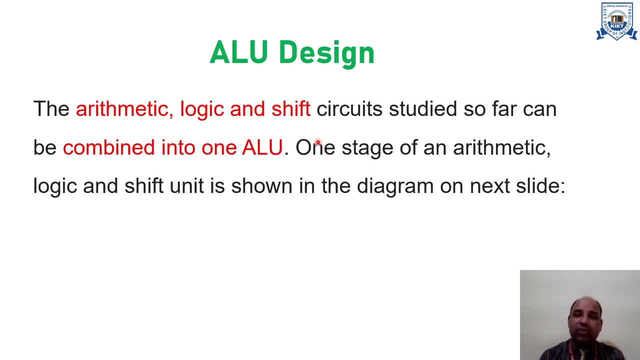 and ultimately, finally, the ALU, which is responsible for converting every instruction of application into the arithmetic and logic and shift operations. so one stage of an arithmetic, logic and shift unit. it is shown in the diagram on the next slide. now let us try to understand how it look likes and how it function. so i move on to the next slide here. 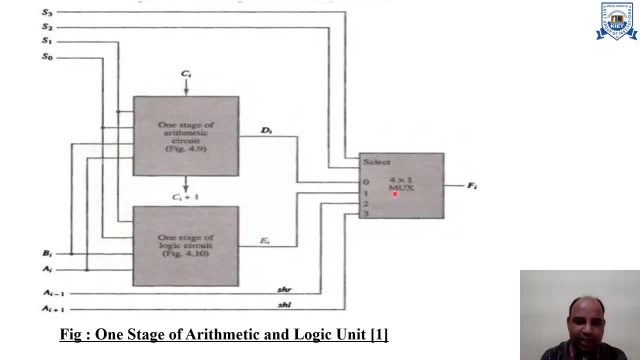 yes, dear friend, this is a very, very complex and important diagram. you can say: and the name is one stage. why i am saying it is just an one stage, or or a partial. you can say arithmetic and logic unit. it is not the complete one, it is, i is just a subscript, if, let us say, 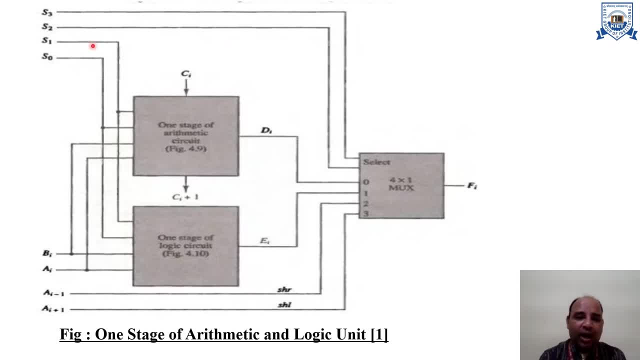 i want to build a and we tell you then i have to include n number of similar stages in my complete alu circuit. then i can say that it is a circuit for the and bit alu. but as i am telling you that designing of the alu and the internal structure of the alu 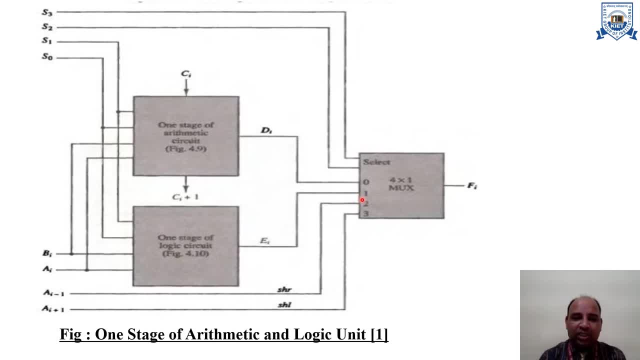 is a complex one. so we are, just for understanding purpose, taking a one stage, only one stage, of the alu. so let us say i say it is decided by the or it is represented by the subscript i. so in this diagram, if you have a closed look on the diagram, it is showing that. 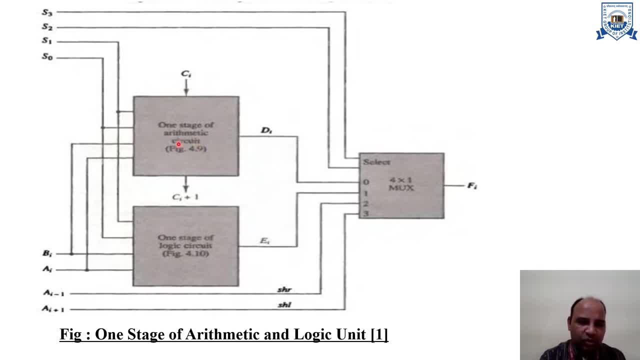 the arithmetic circuit. that is one stage, and repeatedly telling you it is arithmetic circuit here, another is logical circuit. is here then the two box, the two rectangular boxes: one box is showing arithmetic circuit, another is showing the logical circuit, and then finally, there is a four into one multiplexer. now let us try to. 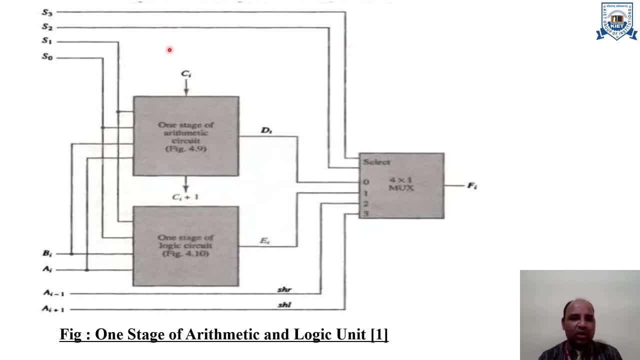 understand how this whole arrangement works. so here as i am telling you that this is the arithmetic circuit and this is the logical circuit. now, the arithmetic and logic circuit. basically this the operations within the arithmetic and logic circuit. they are selected by the use of these two selection lines, which are the s0 and s1. so as you can see here that s0. 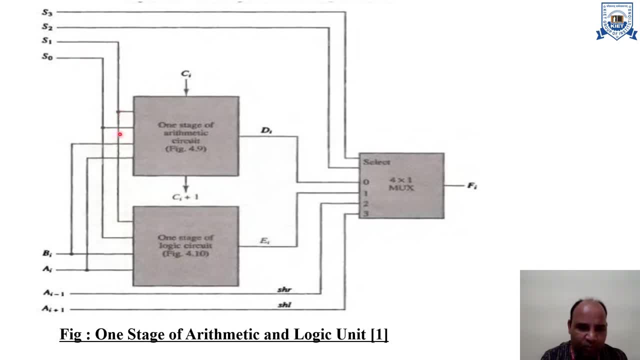 s0 and the s1, both the selection input goes as a, as a input to the arithmetic circuit as well as the logical circuit. and let us say, these are the two numbers, a, i and b, i. these are the two number, a and b, for the stage i, which is represented by the 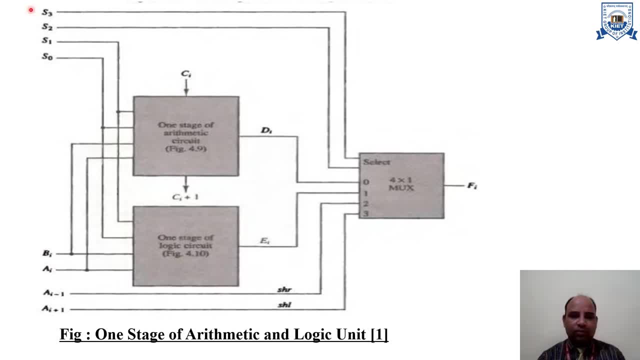 subscript i. so so a and b- they are also goes into the as a input inside the arithmetic circuit and logic circuit means a and b. they also work as a input for this particular logic circuit as well as for the arithmetic circuit. and now one important point is that this is the carry carry from the previous stage. so 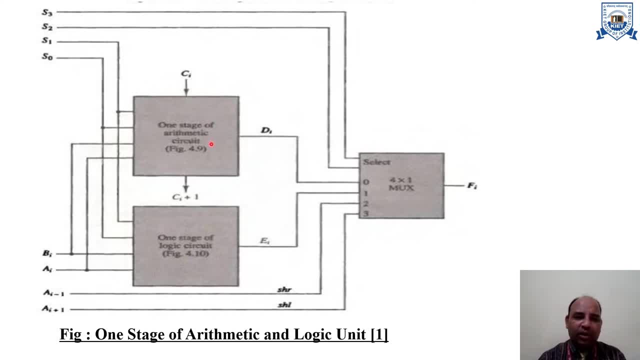 it works. ci works as a input carry to the arithmetic circuit and the next carry, which is out of the arithmetic circuit, ci plus one. it has to be inserted or it must work as a input carry to the next stage, arithmetic circuit. what i mean to say is that it works as a input to the castle creation and now, at the next moment, we get 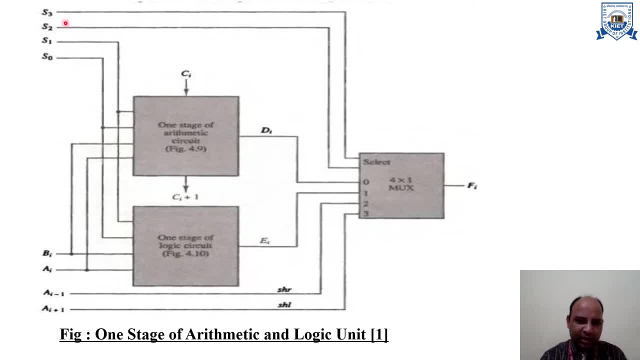 the production line. so we get the production line, that's the cd is now delivered from our code падag. and now and now, moving further, the two selection to another selection line, namely s2 and s3, as you can see here in this diagram. so they are also used in the process, but they work as a input to the multiplexer. 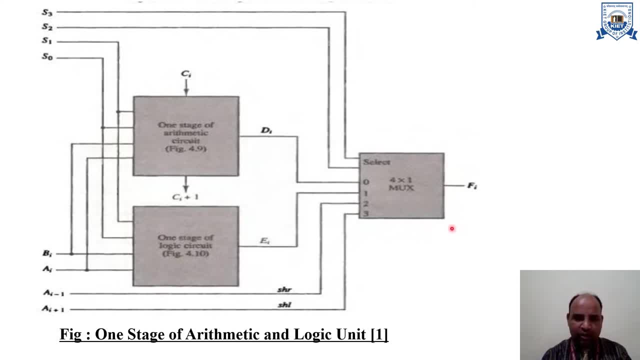 s2 and s3. so as i am telling you that s2 and s3 they work as a input to the four into one multiplexer, with the output passed into the vectoravan multiplexer which is showing in the diagram here. now the important question comes here. that what? 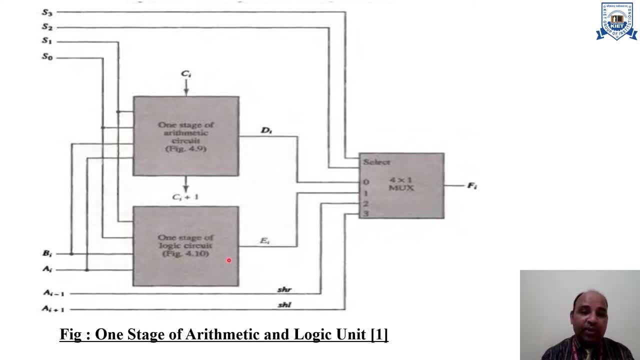 is the purpose of this multiplexer, apart from this arithmetic and logic circuit? so i can tell you that this multiplexer is used to select the output which are coming from the arithmetic circuit. as you can see in the diagram, it is the di air and the ei which is the coming output from. 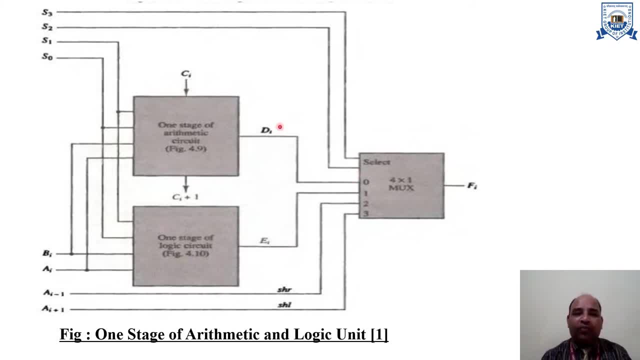 the logical circuit. so basically, for it is used. this particular multiplexer is used for the selection in the two different outputs, with one is from the arithmetic circuit, that is di, and one from the logical circuit, that is ei. one another important line is also here, which is very 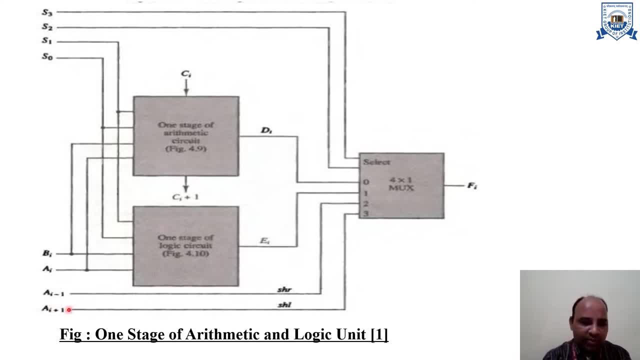 very important point to emphasize here- that ai minus one and ai plus one, these are the two outputs which are coming from the arithmetic circuit. so basically, for it is used are the two additional input. they are also work as a input to this multiplexer. so basically these: 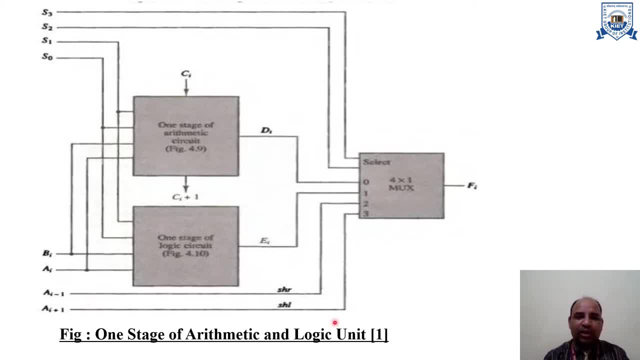 two inputs: ai minus one and ai plus one. they are used for the shift operations. so ai minus one is used for the right shift operations and ai plus one is used for the left shift operation. and finally, fi is the final output of i stage. make sure we are not here seeing the complete structure of the arithmetic. 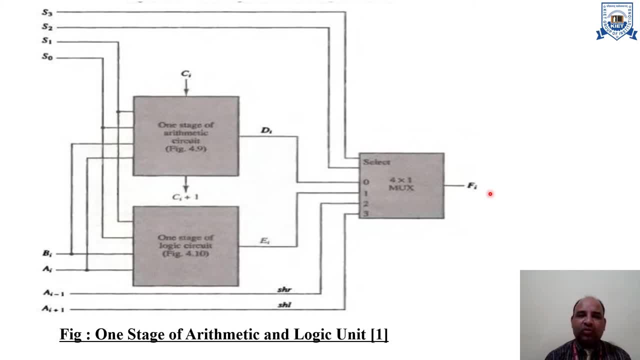 logic unit. as i told you in the beginning of the discussion of this particular alu design that we are just seeing here, the one stage of the alu so fi, i can say that it is the output of this multiplexer, or in other word, it is the output of this particular stage of alu, stage of. 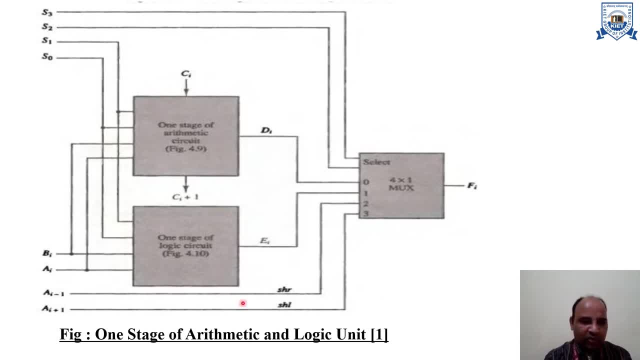 alu. so this is the output of this particular stage of alu. so this is the output of this particular stage, alu. so this is the entire diagram which is showing the internal structure of the one stage of the arithmetic logic unit. and for your kind information again, i am repeating: 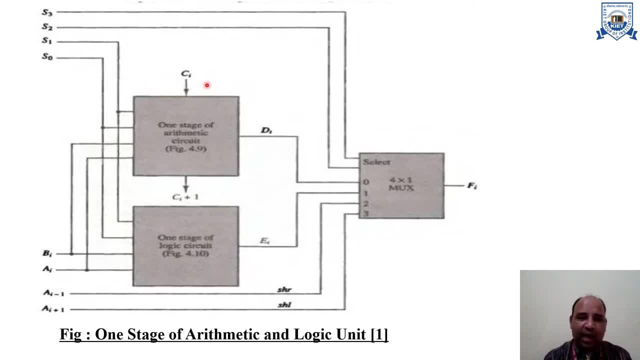 the line that this ci, it is a carry input, and finally then ci plus one, which is the ci plus one, which is the carry output out of the this particular i stage. and now ci plus one will work as a input to the Wohnungstoilς process. and i'm again giving you a brief description. here of the的时候, the monthly interaction in the frame, because possibly this will be an advantage if you don't want to deal with finalization after, to the access given descent. but this, if you do not, I hope that you will save some time. so i am now clear here and now i will. 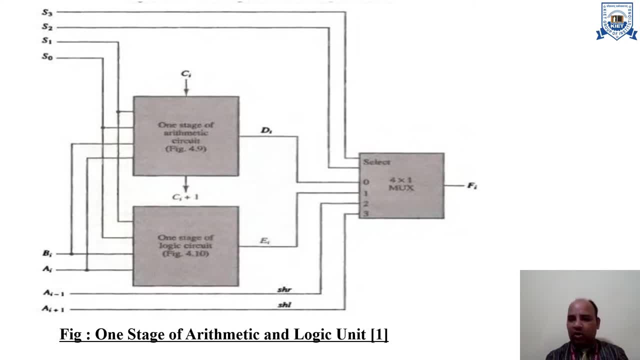 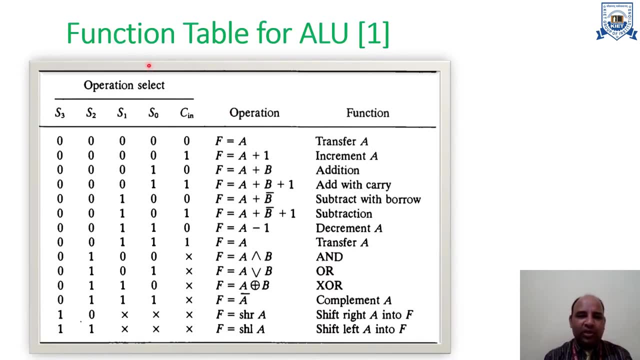 next stage, arithmetic circuit. so now we move on to the next slide from here. dear friend, as you can see on the slide that this is the function table for ALU. so what we discussed just one minute earlier, the a particular stage of arithmetic logic unit. so in terms of function, if I say that arithmetic logic unit of the previous slide, 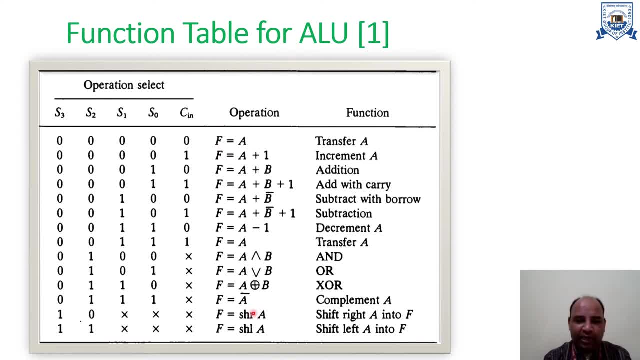 it shows the 14 different operations. what we can see in this function table for the ALU. out of the 14, the 8 are the arithmetic operations up to where, and then from here up to here these are the four logical operation, and then finally these are the two shift operation. so 8 plus 4. 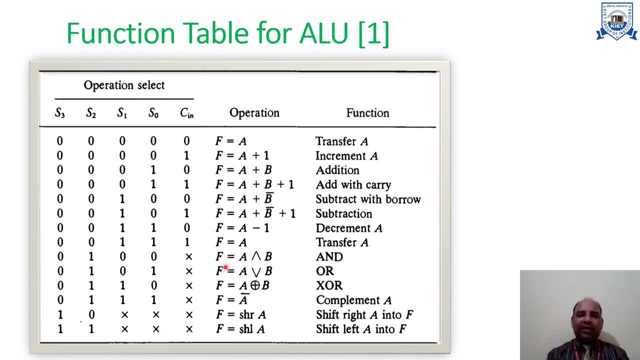 plus 2, what it makes the 14 operation, what is represented by the previous diagram in the previous slide. so as we can see the function table up to this moment, these are the 8. up to this moment, these are the 8. these are the arithmetic operations, so they are generally. 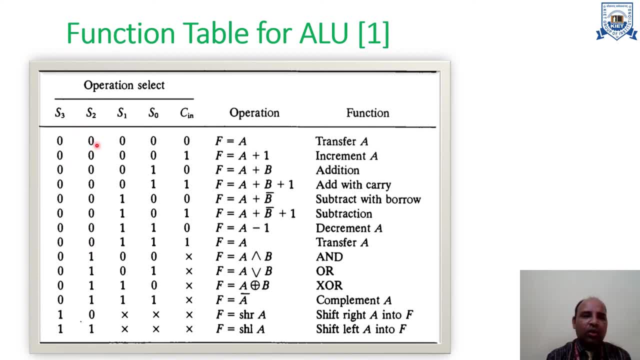 selected when we are having the s3 and s2 both, these selections line, so these are the selection line, what we saw in the previous diagram of the state of ALU. so when these s3 and s2 both are 0 value of these, both input are 0, then we say: all these operations, this, this and up to this they. 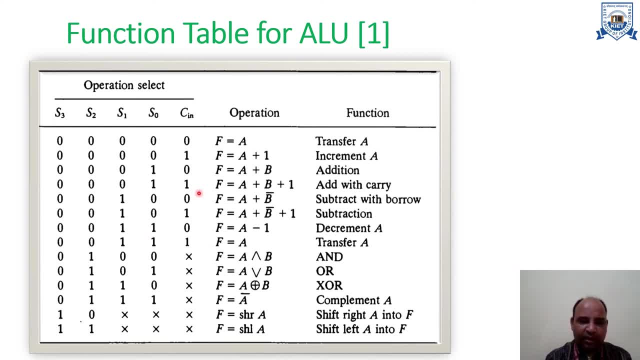 are the arithmetic operations, and here seen plays a very important role in this selection of particular arithmetic. let us say: if it is seen zero, then it is a transfer. F equal to a. if seen is equal to 1, that is increment a. and likewise if seen zero. 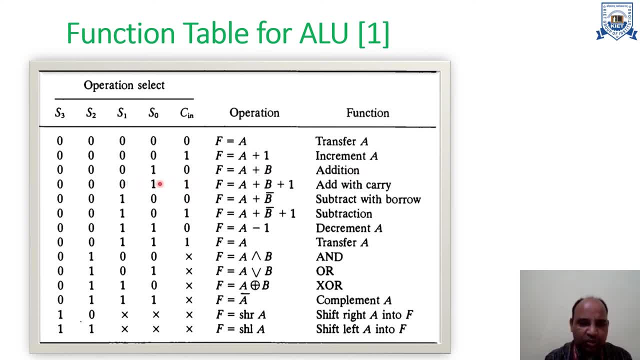 with having s1: 0 and s0 1, it is addition, operation, and similarly, if s1 0, s0 1 and c in 1, it is add with carry, which is f, a plus b plus 1. so in nutshell i can say that, up to this list, when s3. 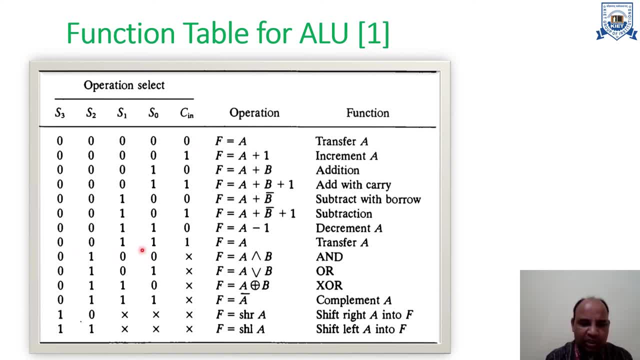 s2. both are 0. so the selection of a particular arithmetic operation is done with the help of s1 input, s0 input and the carry input that is c in now goes down to the list. when s0- sorry- s3- is 0 and s2 is 1, it is s3 0 and s2 1. so 0, 1, 0, 1, 0, 1 and 0, 1. these four are represented as the. 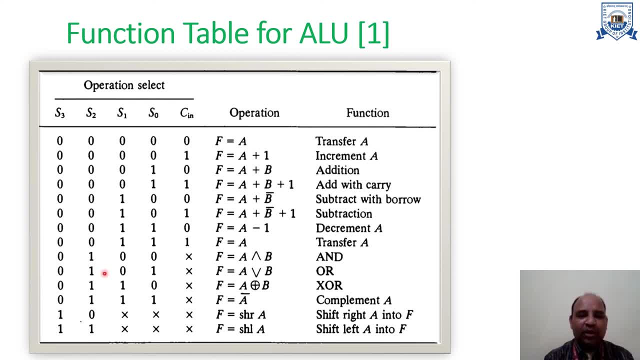 logical operation when the value of s3 0 and s2 1, so for this entire space. these represented as the logical operation, so for this entire space. these represented as the logical operation, so for this entire space. these represented as the logical operation and individual logical operations. make sure they are only represented or they are only. 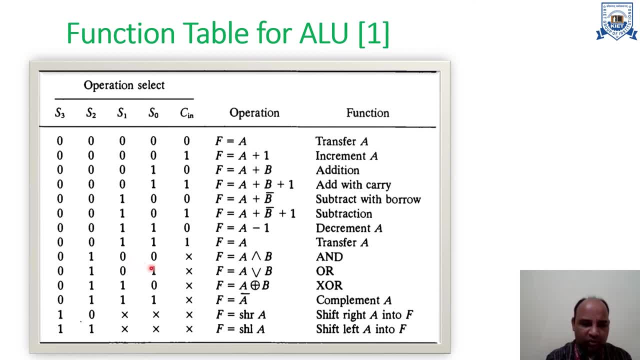 categorized with the help of the selection line s1 and s0: s1 and s0: when both are 0, then it is a logical, and when s1- s0 is 0- 1, it is a logical. or and when s1 and s0 is 1- 0, it is a logical xor. 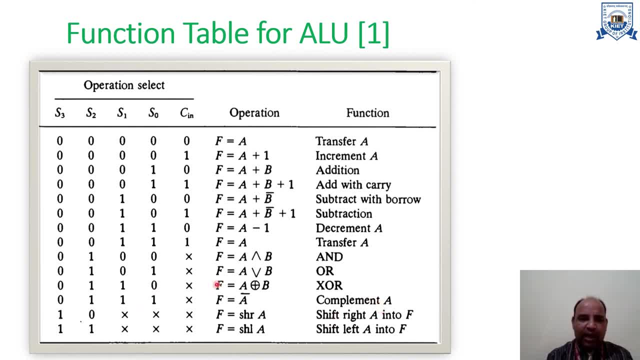 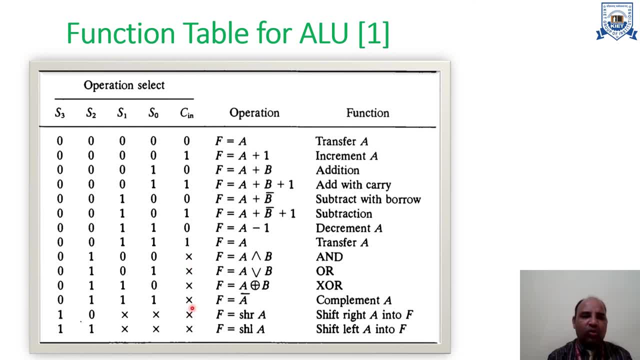 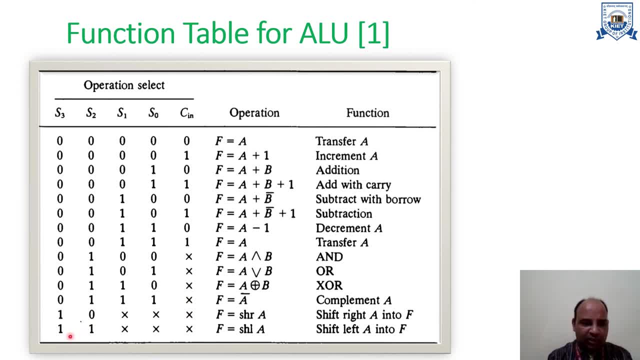 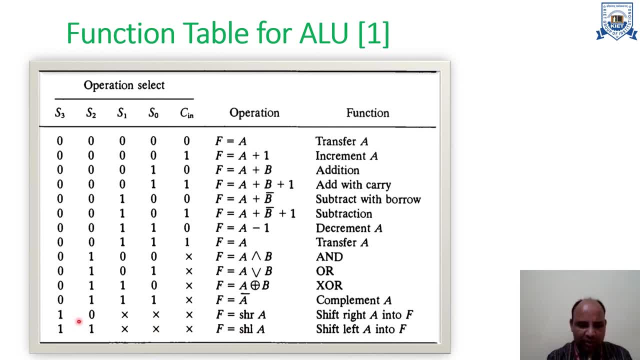 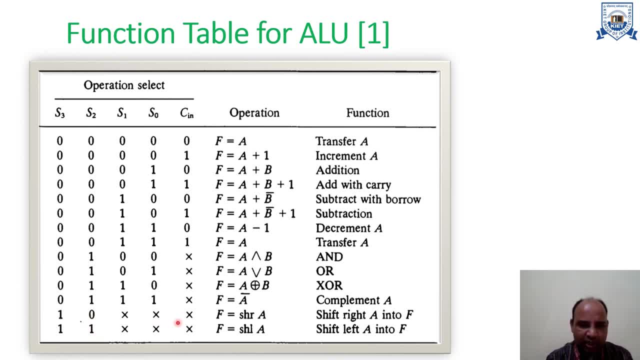